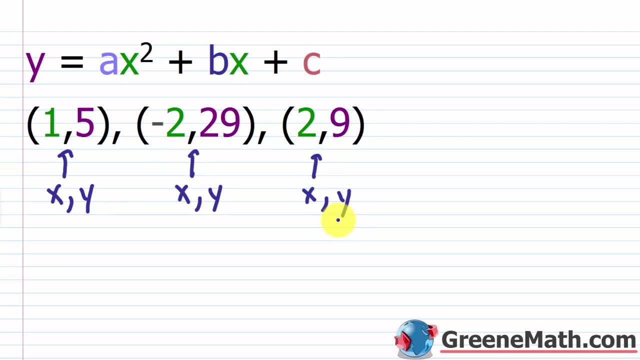 is pretty easy to do. All I'm going to do is set up three equations, okay, so that I can solve for the three unknowns- The three unknowns are going to be the a, the b and the c here that I'm going to need to write this equation, Okay. so what I'm going to do? I'm going to rewrite this, let's just. 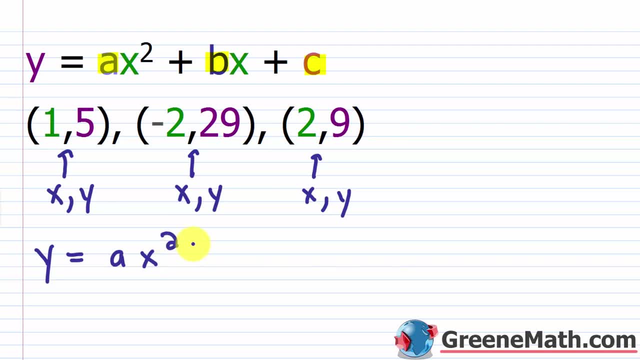 say it's y equals. we've got ax squared plus bx, squared x plus c, and what we're going to do is we're going to plug in for x and y. We're going to do that three times. So let me erase this and let me just put some parentheses, and I'm just going to. 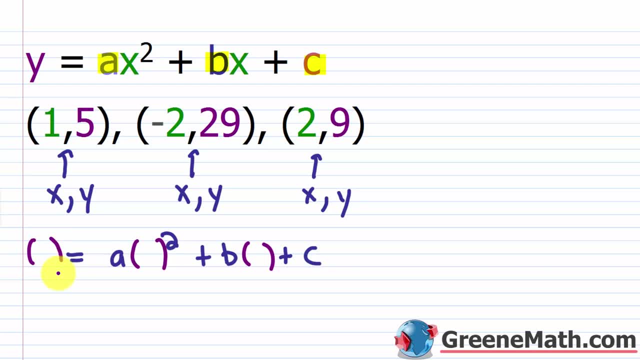 be doing some plugging in and let me erase this and put some parentheses and, to make this really easy, I'm going to highlight where I'm plugging in x with a yellow, okay, and I'm going to highlight where I'm plugging in a y with a kind of blue. Maybe it's a light blue, I'm not sure. the official 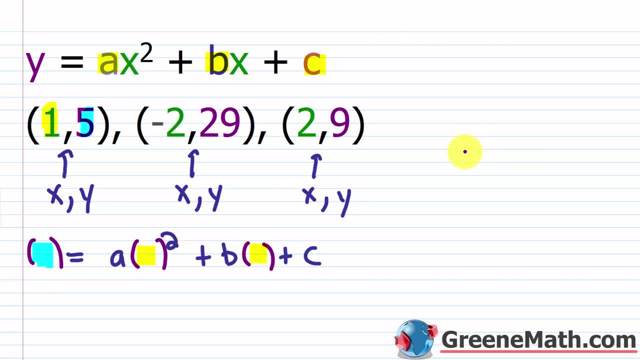 color on that. so let me highlight that. I'm going to highlight this and then let's go through and do this. So y gets plugged in here right, because it's y equals ax squared plus bx plus c. So y is all the way to the left. so I'm 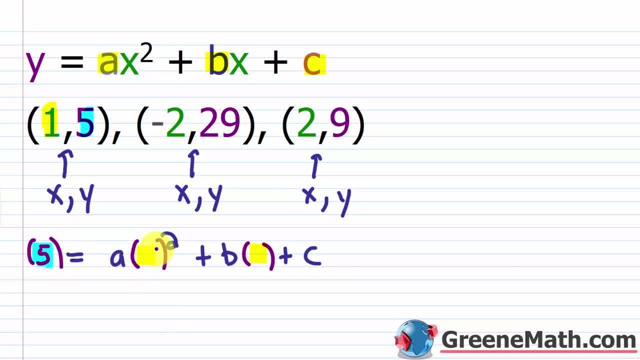 going to plug a five in there, Then this equals: we have a times. there's an x that goes in here, so that's going to be one, and then that's squared. then plus b times. again you have an x that goes there, so that's going to be a one, and then plus c. Okay, so that's your first equation. So for this, 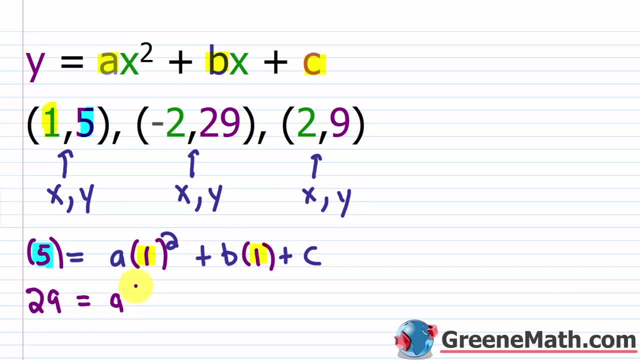 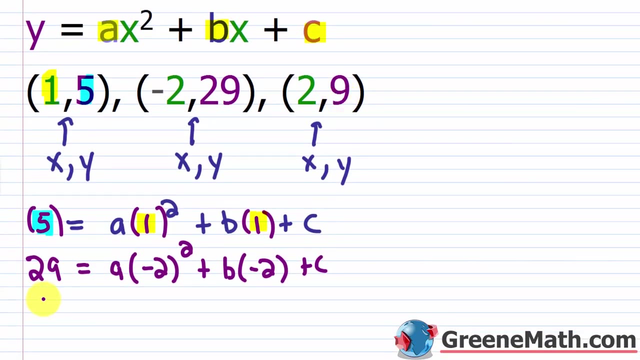 guy. it's going to be 29 for y and it equals a times in my parentheses. I'd have negative two and that's squared, and then plus b times. again I'm going to have negative two and then plus c, And then for my third equation, my final equation, again I do the same thing. So y is nine, so nine. 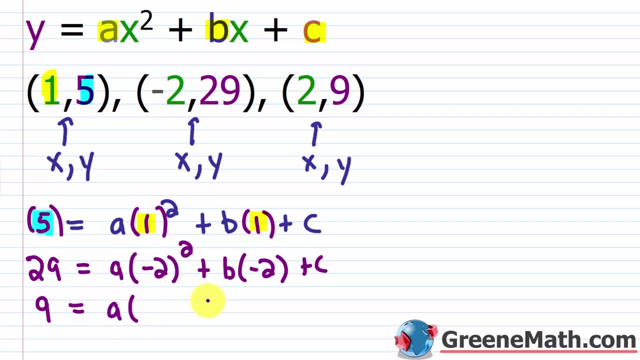 is going to go out here and this equals: you have a times in the parentheses. I'm going to have a two, this is squared, then plus b times. again, I'm going to put a two and then plus c. So let's copy this real quick and let's go to a fresh sheet so we have some room to work. Okay, and I'm just going. 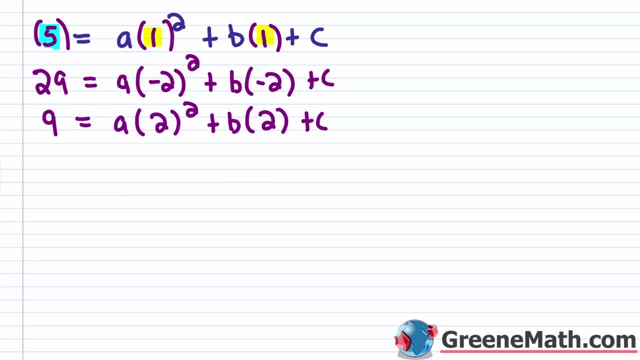 to rearrange this a little bit. So I'm going to simplify some things. so I'm going to say equation one: I know that one squared is one, so this would just be a, and then plus b times one is just b and then plus c, and this equals. we have. 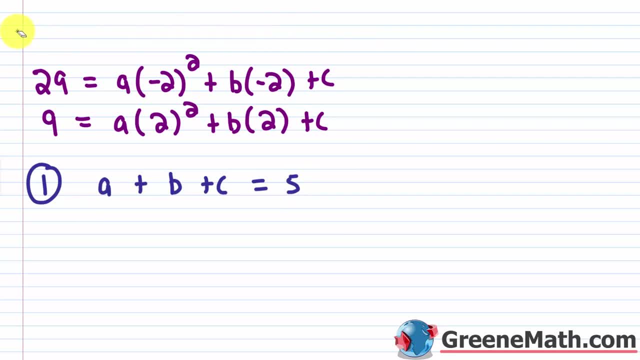 five. Okay, so that's my equation one. so let me just erase this from here, I don't need it anymore. and then for equation two, I have negative two squared, which is four, then times a, and then plus negative two times b, so I can just put minus two b, if you want, and then I have plus c and of course, 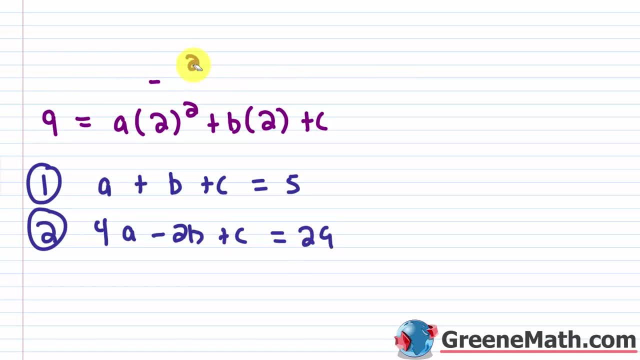 one is equal to twenty nine, and so let's erase this. we're done with that. and then now for equation three. I have this guy: two squared is four, then times a, and then I have two times b, which is two b. so plus two b, and then plus c, and this equals nine. So I have my three equations, three unknowns. 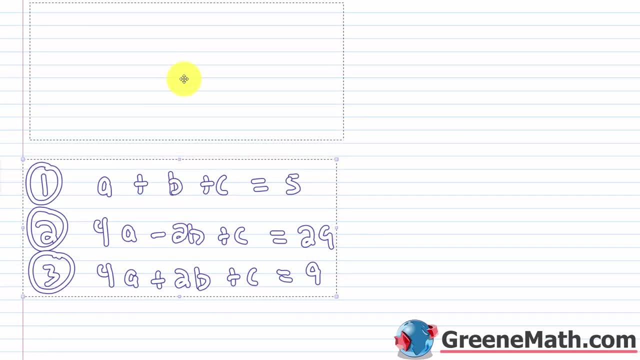 pretty easy to solve for this. So let me scooch this up and let's get started. Alright, so we know from the last lesson that all we need to do is take kind of two equations from one to two. we can just draw a line from this up and run it through it. Now let's take the first of each of the two numbers and then the second of the two numbers, and four of them are the same numbers. 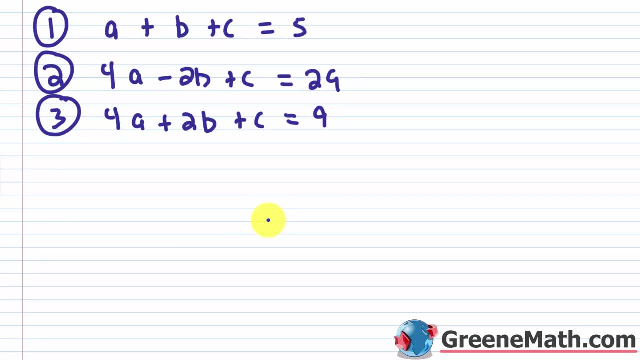 Okay, so let's make this a number and let's keep it like that. this is the one and this is the three, six, two equations from this system. pick a variable and eliminate it. Okay, That's how we kind of get the ball rolling, And what I want to do I'm going to look at equation one and two. It's probably. 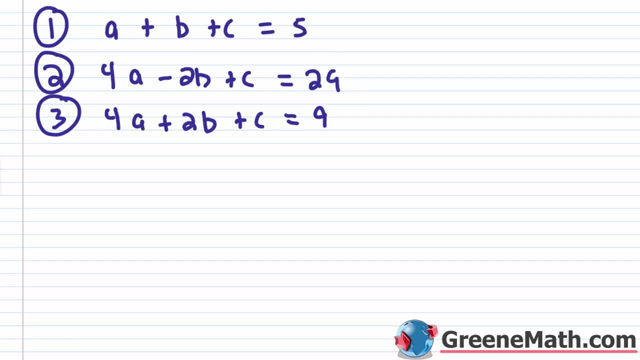 easiest here to eliminate C, Okay. So what I'm going to do is I'm going to multiply equation one by negative one, Okay, And then I'm going to add that to equation two. Okay, Because what I'm going to do, if I multiply equation one by negative one, this is going to end up being a negative C. 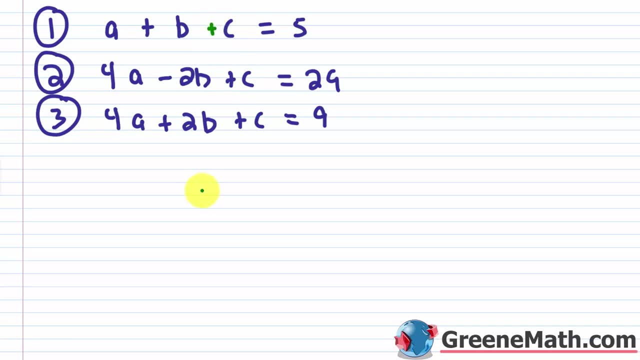 there, Okay. And then negative C and positive C. those are going to cancel All right. So negative one multiplied by equation one would be negative. A minus B minus C equals negative five. Okay, I just multiplied everything by negative one, So it just changed the sign of each term. That's all it. 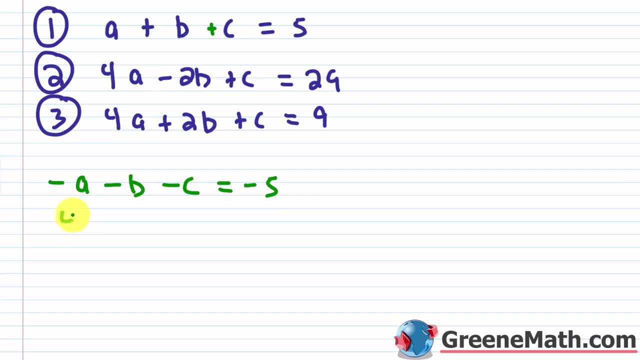 did. And then for equation two, we keep that as it is. So 4A minus 2B plus C equals 29. And then we're going to add these two equations together. So remember, when we do this, we're adding the two. 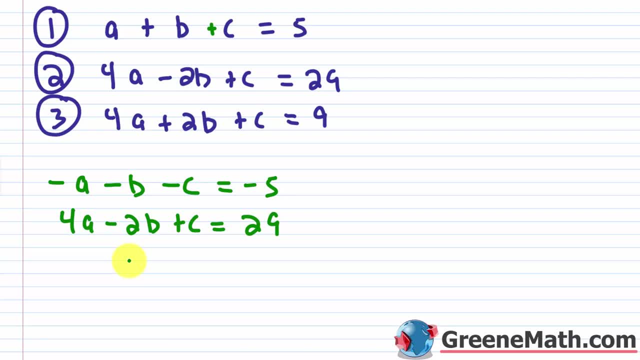 left sides together. So we're going to add these two equations together. So we're going to add these two equations together And we're setting this equal to the sum of the two right sides. Now, in order for this to work, you have to have your equations in the format where the variables you're 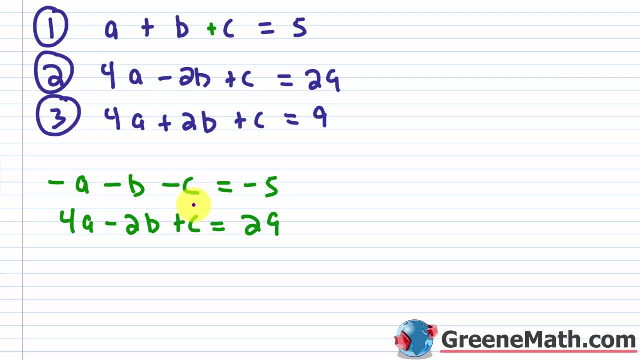 working with are on one side and the number, the constant, is on the other. Okay, So you see how I have all my variable terms, my terms, with the A, the B and the C involved. that's all on the left and the constants on the right. So you want to set it up that way? All right. So if I add negative A, 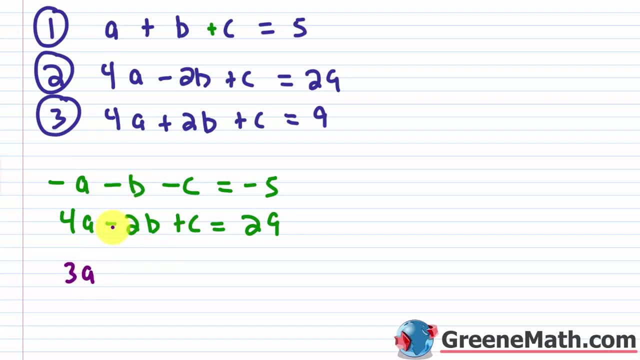 plus 4A, I'm going to get 3A, Then negative B plus negative C equals 29.. And then I'm going to add: negative 2B would be minus 3B, Then negative C plus C. we know this would cancel And this: 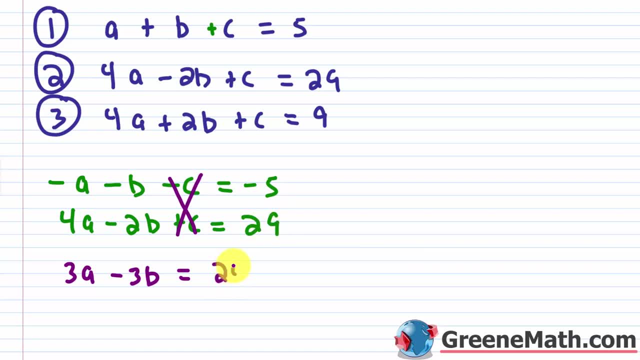 equals negative. 5 plus 29 would be 24.. So let's call this equation 4.. And I'll say: this is 3A minus 3B is equal to 24.. So let's erase all this. We don't need any of this anymore. 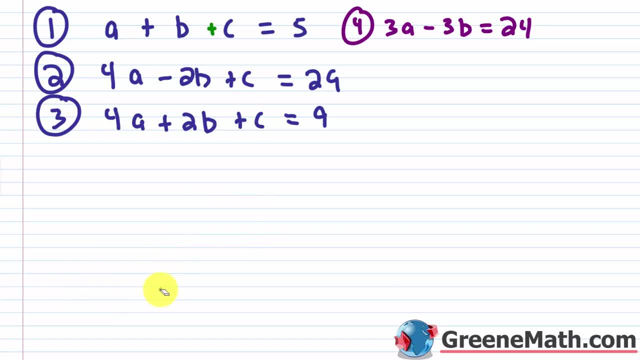 And now let's pick two other equations. It can't be 1 and 2, because we already used those. So any two other equations we could do 1 and 3, or 2 and 3. And we want to eliminate the same variable. So we want to eliminate C again And that's pretty. 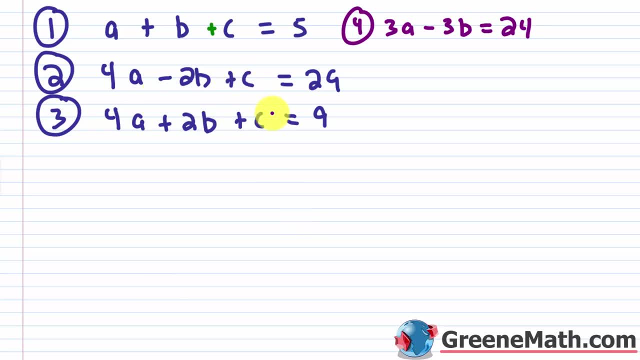 easy to do. So if I pick 2 and 3, let's just go with that. If I multiply equation 2 by negative 1, I'd have negative 4A plus 2B minus C equals negative 29.. And then for equation 3, I'll just 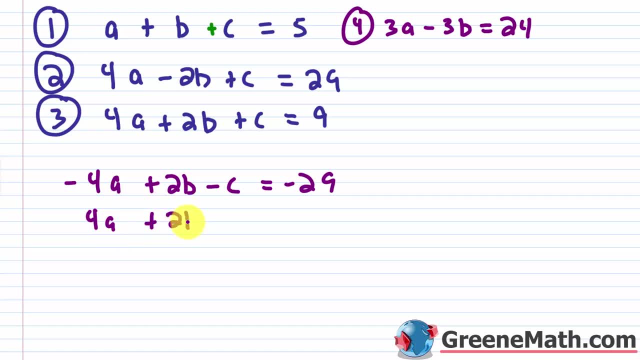 keep it as it is, So 4A, and then we're going to have plus 2B, and then plus C, and this equals 9.. Okay, So when we do this, we get an even easier situation. This is going to cancel, and so is 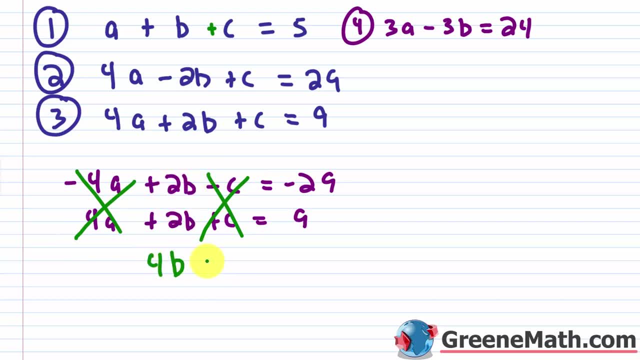 this. So I get 2B plus 2B, which is 4B, And this is equal to negative. 29 plus 9 is negative 20.. So for equation 5, I get: 4B is equal to negative 20.. And let me erase this real quick. 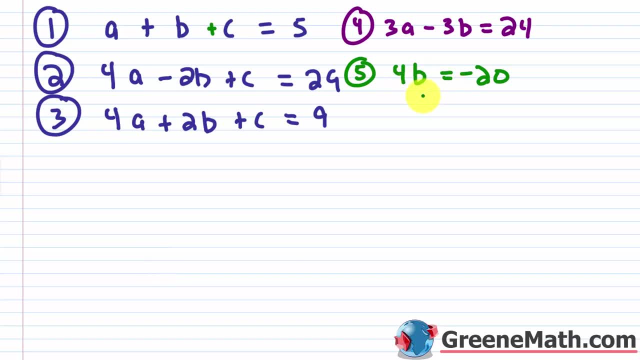 This one just happens to be much easier to work with. If I divide both sides by 4, I find that B is equal to negative 5.. Okay, So I've already got one value: B is negative 5.. I can plug that back in here in equation 5.. 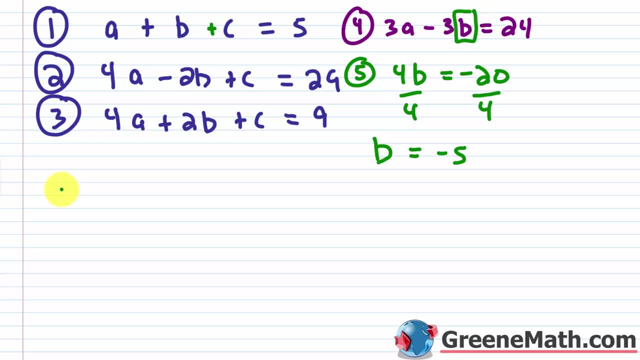 And I can figure out what A is. So I would have 3A minus 3 times plug in a negative 5 for B, So plug in a negative 5 there And this equals 24.. Okay, So what we'll do? we have 3A. 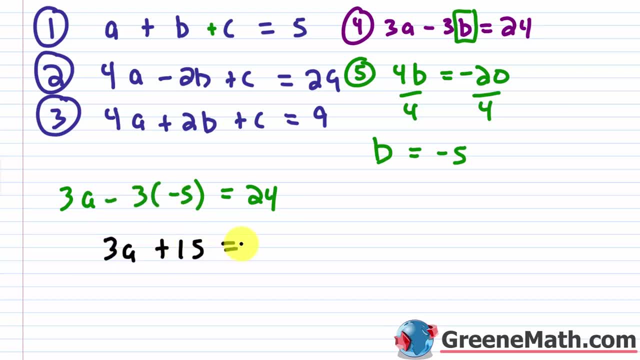 and then negative 3 times negative. 5 is plus 15. And this equals 24.. Okay, So if I subtract 15 away from each side of the equation- let me kind of do this up here- We're going to have 3A- is. 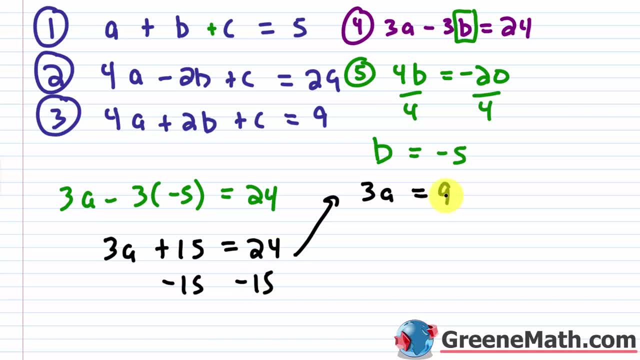 equal to 24 minus 15 is going to be 9.. And then we're going to have 3A plus 15 is going to be 9.. Divide both sides by 3.. And we find that A is equal to 3.. Okay, So my board's getting kind of. 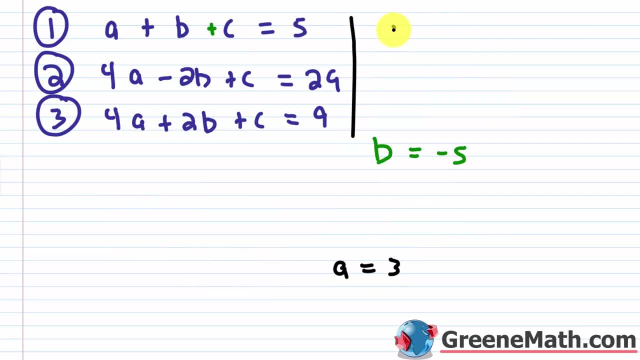 busy, So let me erase some stuff. So at this point I know that A is equal to 3 and that B is equal to negative 5.. So what is C? C equals what Well, I can find C by just plugging back. 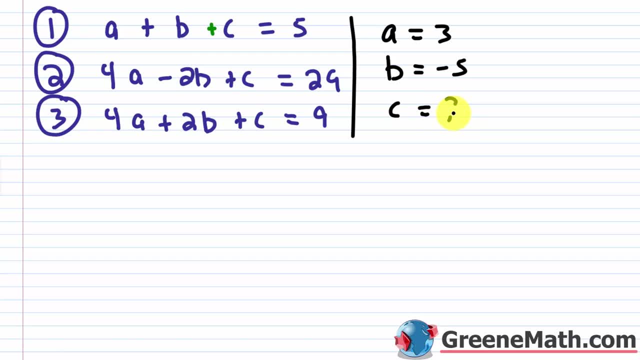 into either equation 1,, 2, or 3.. It's easiest to work with equation 1.. So let me plug in a 3 for A and a negative 5 for B. What would that give me? So you would have 3 plus negative. 5 plus C equals 5.. 3 plus negative 5 is 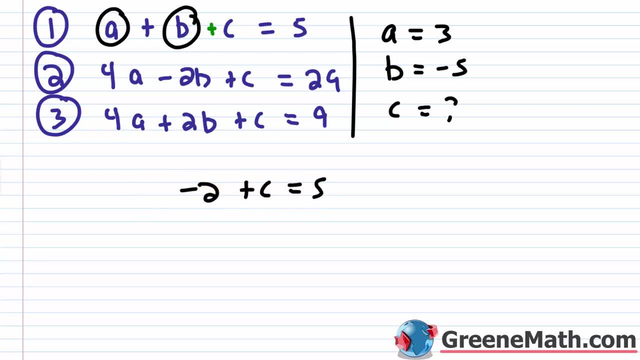 negative 2.. So you'd have negative 2 plus C equals 5.. If I add 2 to both sides of the equation, I get C is equal to 7.. So now I have enough information to write the equation of this parabola in standard form. So let me just copy this and go back up. So we have that A is 3,. 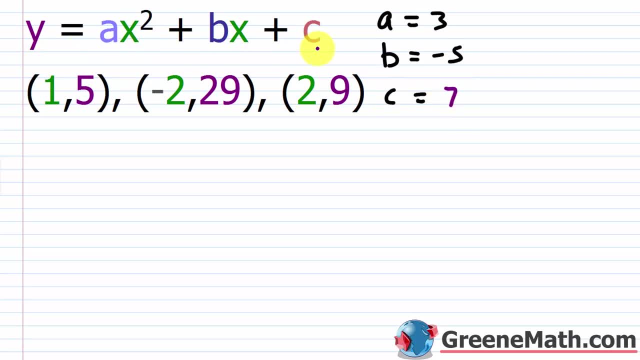 B is negative 5, and C is 7.. So just plug into your standard form and you'll see that B is negative 5.. We have Y is equal to for A. I'm going to put a 3, and then times X squared. 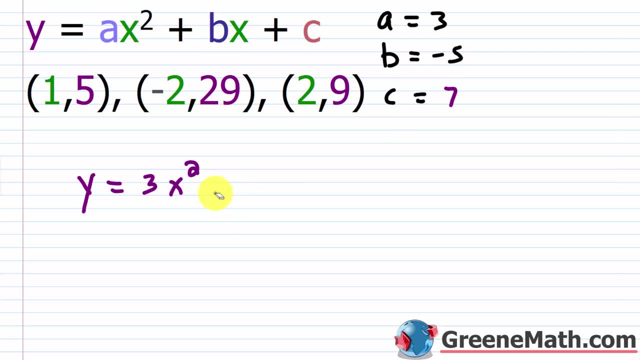 then plus, Then for B it's negative 5.. So instead of plus let me just put minus 5 here, and then times X, and then plus C, and C, of course is 7.. So the equation is: Y equals 3X. 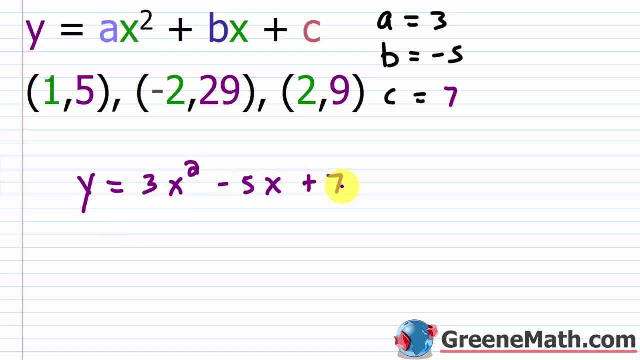 squared minus 5X plus 7.. If you wanted to check this, you could plug in for X and Y and verify that you get a true statement in each case. I've already done this. I know that it works out, But again, just to do one of them, you could plug in a 1 for each X and a 5 for the Y. 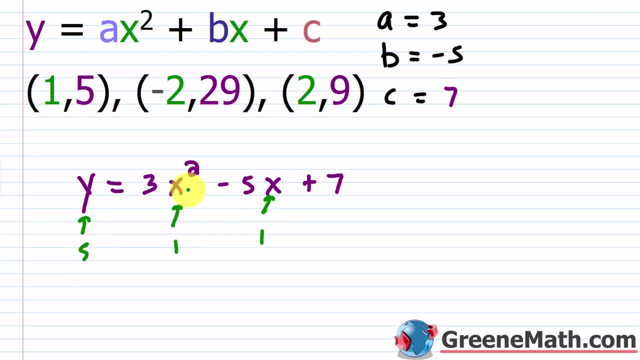 and verify, you get a true statement. 1 squared is 1.. So 1 times 3 would be 3.. And then 5 times 1 is 5.. So minus 5 plus 7.. 3 minus 5 is negative, 2.. Negative 2 plus 7 is 5.. So we would have 5 equals. 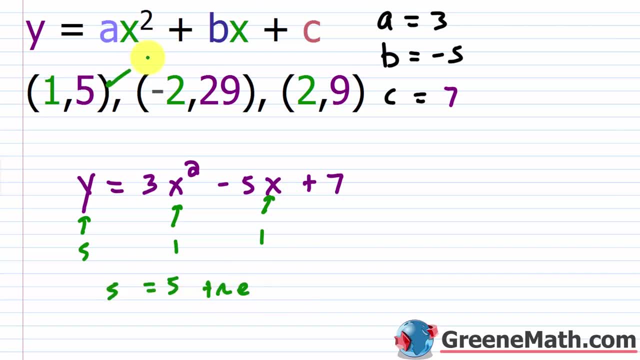 5, which is true. So we know this one works. Again, I'll leave it up to you to check these other two, But I can tell you right now you're going to get a true statement. So you're going to get a true statement. 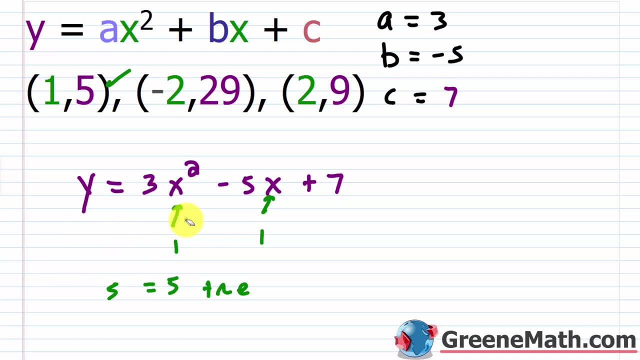 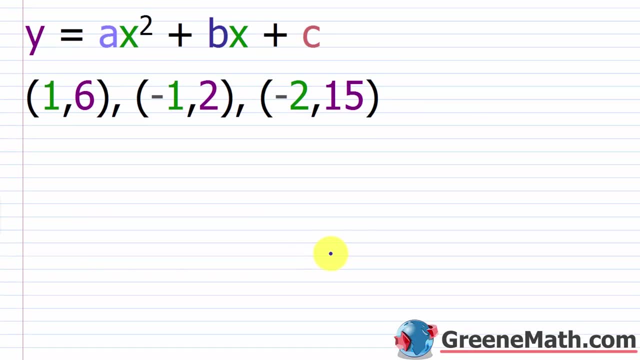 I've already checked them and they do work. So our equation is going to be: Y equals 3X squared minus 5X plus 7.. All right, so let's look at another example. So again, we have our Y equals. 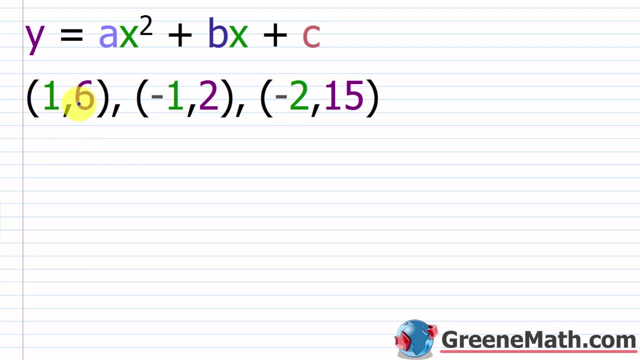 AX squared plus BX plus C. And now we're given the points 1 comma 6, negative 1 comma 2, and negative 2 comma 50. So again the same process. We're going to say that Y is equal to AX squared. 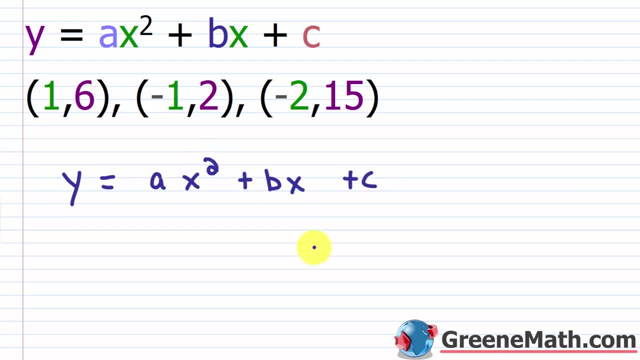 plus BX, plus C, And we're just going to plug in for X and Y. So we're going to plug in for X and Y again using this data from the points. So for the first one, again, if I'm plugging in for X, 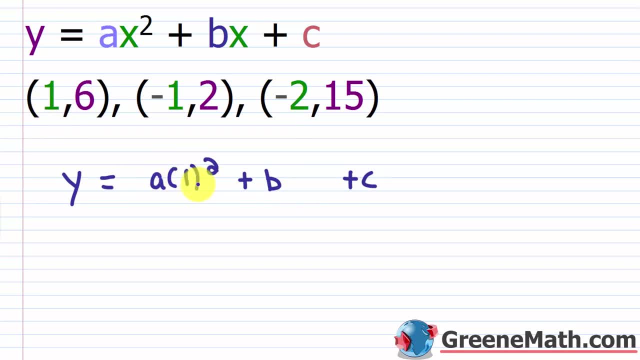 we have an X comma Y. The X is 1.. So that's 1. And the Y is 6.. So let's put a 6 there. Then for the next one you would have a 2 for your Y And then your X would be negative 1.. 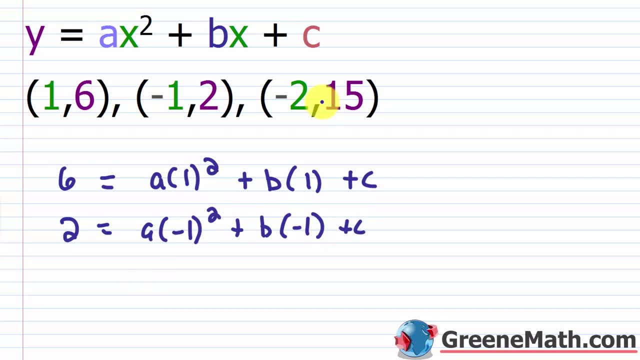 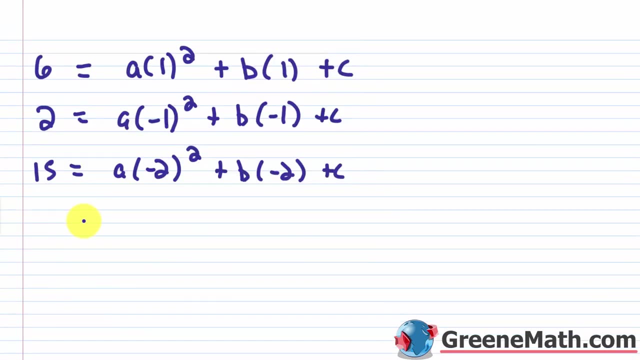 OK, so let's fill that out. And then, for the last one, your Y would be 15. And your X would now be negative 2.. OK, so let's copy this and go to a fresh sheet. OK, so let's go ahead and make sense of this real. 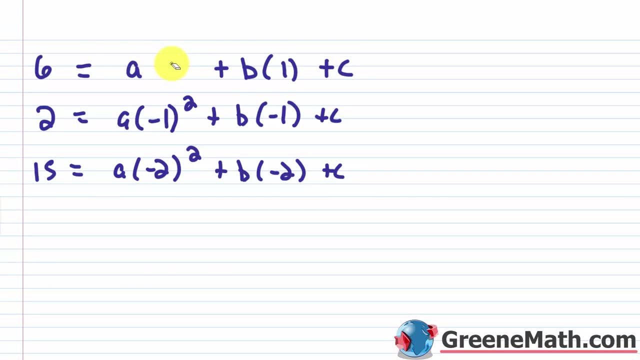 quick. So 1 squared is 1.. 1 times A is just A, 1 times B is just B. So that's fine like it is. So we would have A plus B plus C And let's just put equal 6, like this, And I can clean that up. 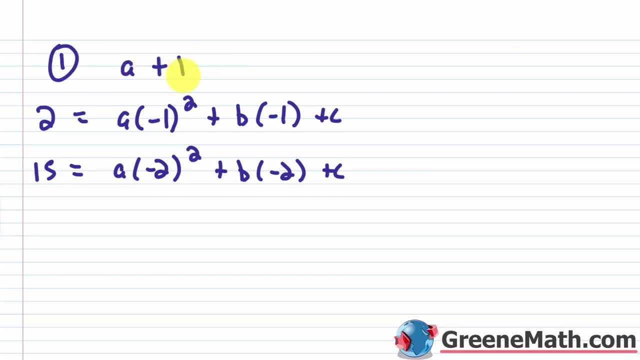 and make it look a little nicer. So for 1, we have: A plus B plus C equals 6.. All right, for this second one, negative 1 squared is 1.. 1 times A is just itself Negative. 1 times B would just be. 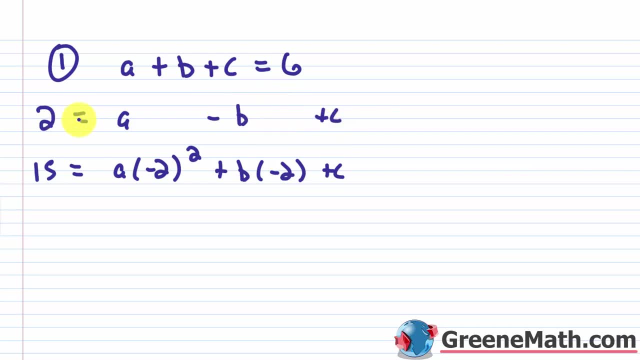 minus B, And then you have plus C And of course you have this equals. You have this 2 over here. So let me move that over here. We'll say that A minus B plus C- A minus B plus C- is equal to 2.. So this: 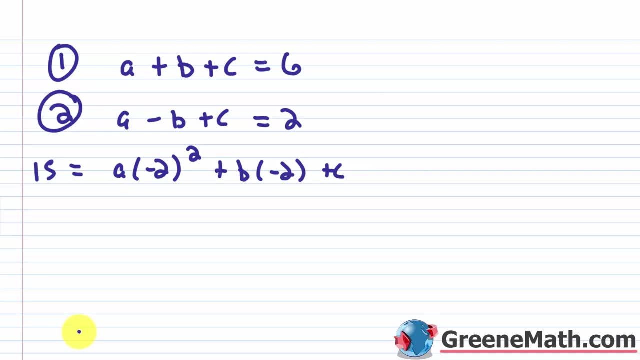 would be my equation 2.. OK then for equation 3, we have negative 2 squared, which is 4.. So this would be 4A. You have negative 2 times B, which is minus 2B, So minus 2B, And then you just have. 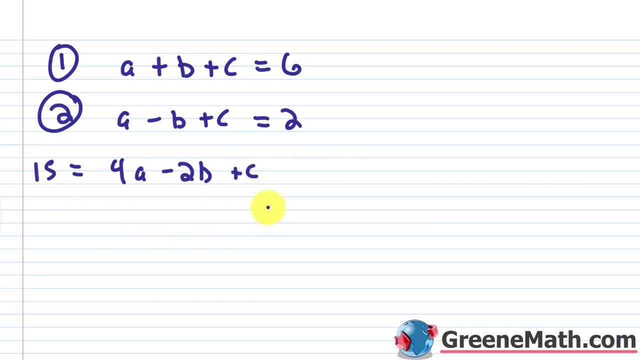 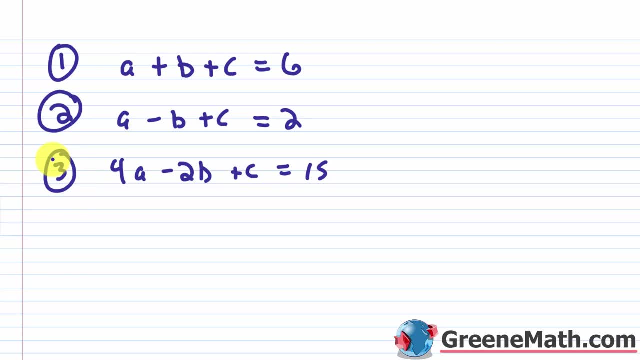 3. OK, so we can just pick a variable to eliminate. Again, you can do C, B or A, whatever you want to do. C looks like it's pretty easy. You have a coefficient of 1 in each case. B is also pretty. 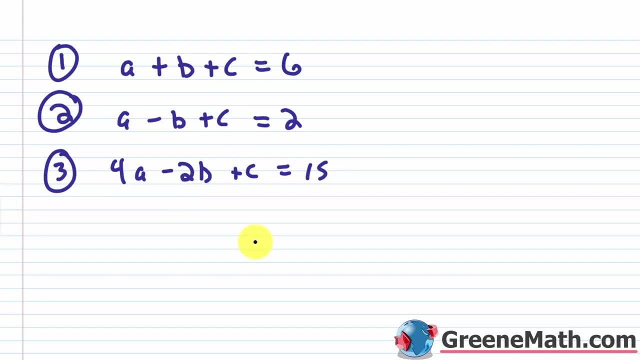 easy as well. So let's just use B to kind of change things up. So if I eliminate B from using equation 1 and 2, what I would do is just add 1 and 2 together, right, because I have opposite. 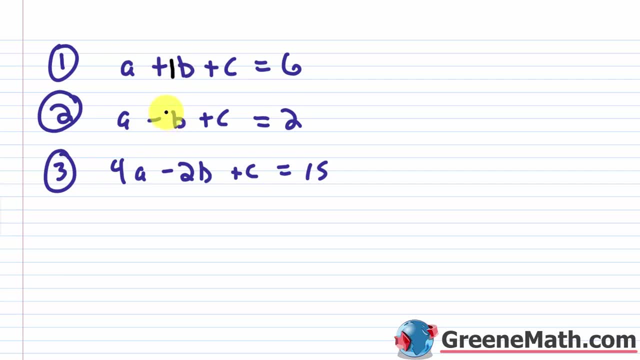 coefficients on B here and here: right. So I have a 1B and a negative 1.. So I have a 1B and a negative 1B there. So I'm going to just add the two equations together and get equation 4.. So A? 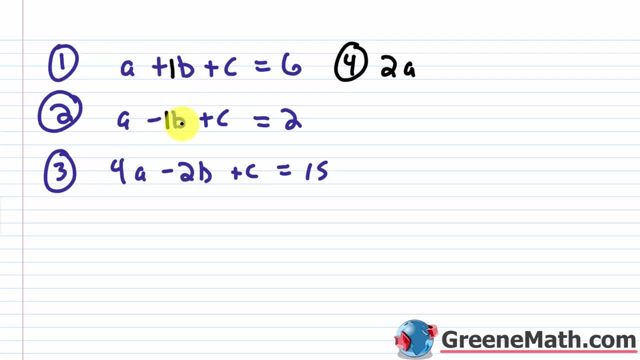 plus A is 2A, And then 1B plus negative 1B. that's going to cancel C plus C is 2C. So plus 2C, And this equals 6 plus 2 is going to be 8.. Now I can simplify the equation, because everything's. 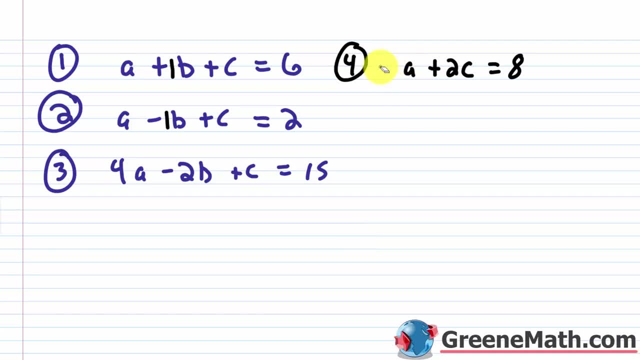 divisible by 2.. So if I divide 2A by 2, I get A, If I divide 2C by 2, I get C, And if I divide 8 by 2, I get 4.. So A plus C equals 4.. 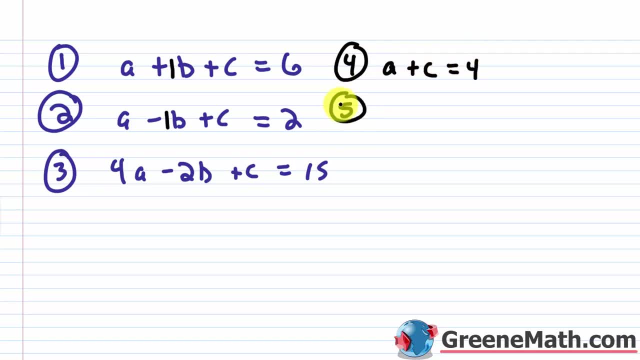 All right for equation 5,. let's just go through and get this from equation 1 and equation 3,. okay, So I'm going to multiply equation 1 by 2.. So I would get 2A plus 2B plus 2C equals 12,. 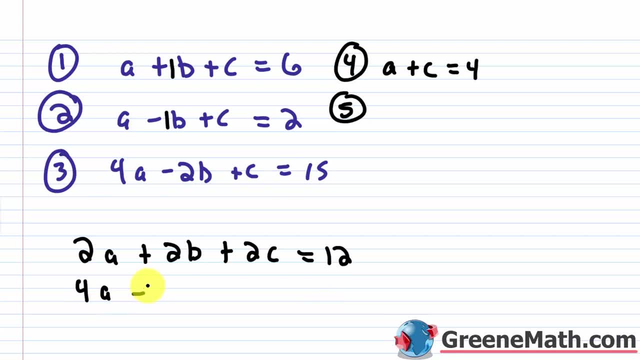 okay, And then for equation 3, I'm going to leave it as is. So 4A minus 2B plus C, and this equals 15, okay, So the reason I multiplied equation 1 by 2 is so I can have. 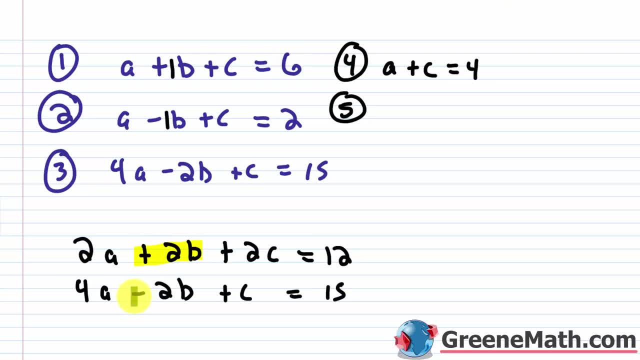 opposite coefficients here, S2, and S3.. So if I divide 2B plus 2C, I get 2A plus 2C equals 4.. To: i've got a plus 2b and i've got a minus 2b. okay, so those are going to cancel. so 2a plus 4a is. 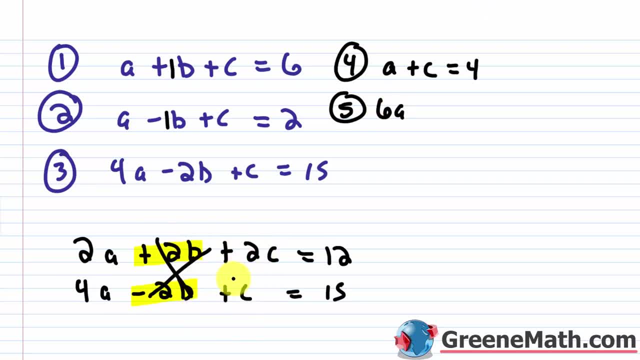 going to give me 6a. these again are going to cancel. 2c plus c is going to be 3c, and then 12 plus 15 is going to give me 27. okay, now, each part here is divisible by 3. 6 divided by 3 is 2. 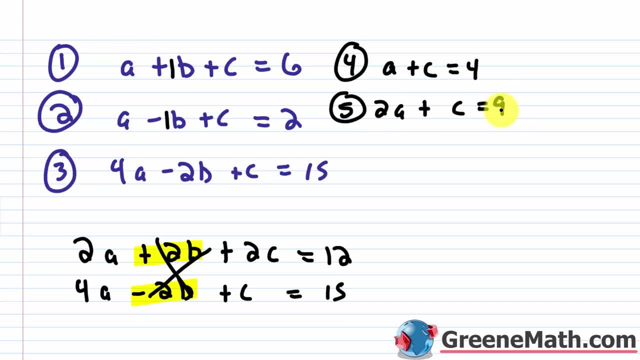 3 divided by 3 is 1. 27 divided by 3 is not okay, so let's erase this. now we can solve this system pretty easily, either using substitution or elimination. let's just use substitution. that looks pretty easy. so i'm going to solve equation 4 for a. so i'm going to say that it's a is equal. 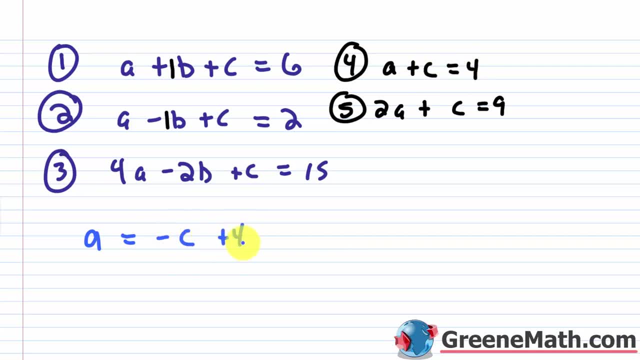 to subtract c away from each side of the equation. so negative c plus 4. i'm going to plug in for a in this equation 5. okay, so this right here, that's what a is equal to. that's what i'm going to plug in for right there. so i would have 2 times this quantity here: negative c plus 4. okay, just plug. 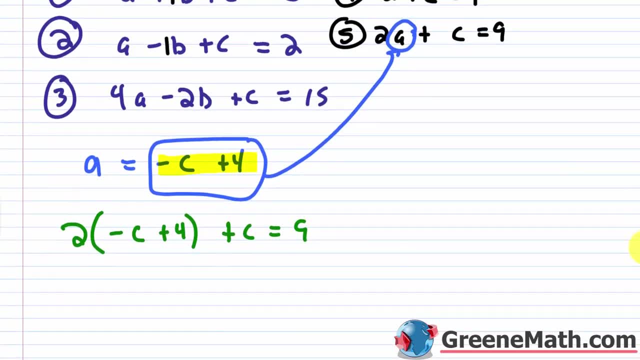 it in and i'm going to plug it in, and i'm going to plug it in, and i'm going to plug it in and in. there then plus c equals 9.. Let me scroll down real quick and get some room. So 2 times negative. 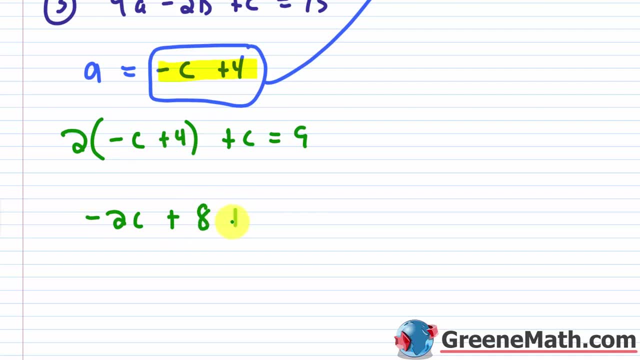 c is negative. 2c plus 2 times 4 is 8. then plus c equals 9.. Negative 2c plus c is going to be negative c, and then plus 8 equals 9.. Subtract 8 away from each side of the equation You can. 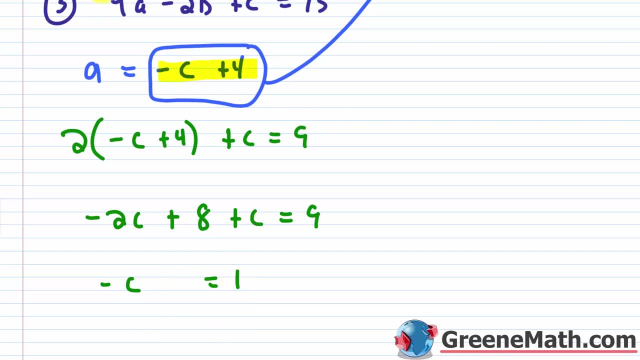 basically just erase it here and just say: this is a 1.. So to finish this up, we can divide both sides by negative 1 and we'll find that c is equal to negative 1.. So that's our answer for c. So let me. 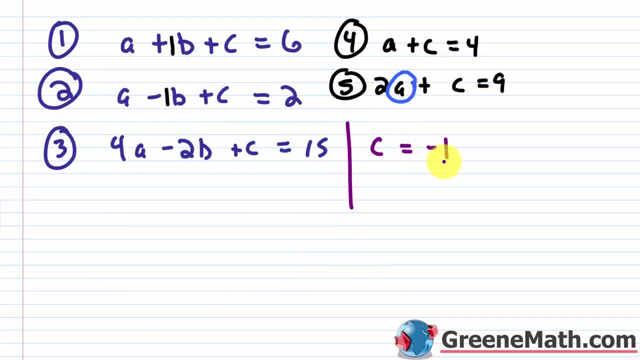 erase all this. So I'm going to say that c is equal to negative 1, and then I can plug in for equation 4 or 5, doesn't matter. Figure out what a is. So let me use equation 4, because it's a. 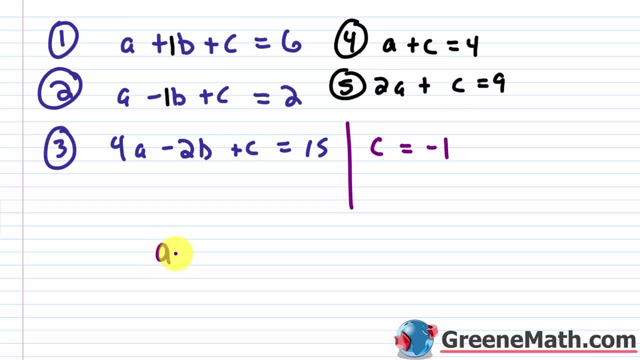 little bit easier. If I plug in a negative 1 for c, I'd have a. you could basically say: minus 1 equals 4.. Add 1 to both sides and you'll find out that a is equal to 5.. So now we have c and we have a. We need to find b. Okay, so b is still unknown. I can get rid of. 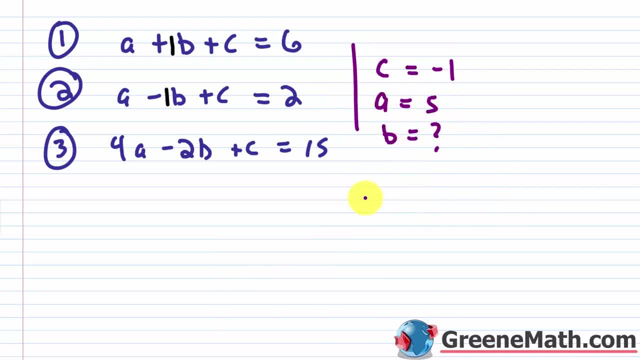 this. I don't need that information anymore. Let me scooch this up, and so what I'm going to do is plug into again either 1,, 2, or 3. Doesn't matter. Figure out what b is. So the easiest equation looks: 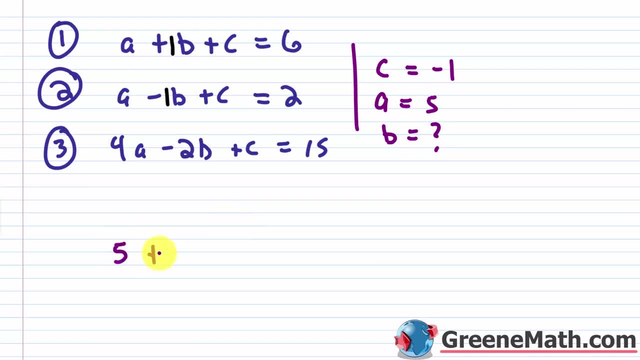 like equation 1.. So I have an a value of 5 plus b plus a c value of negative 1.. So let's just write minus 1 and this equals 6.. So 5 minus 1 is 4.. So we'll say that this is b plus 4.. 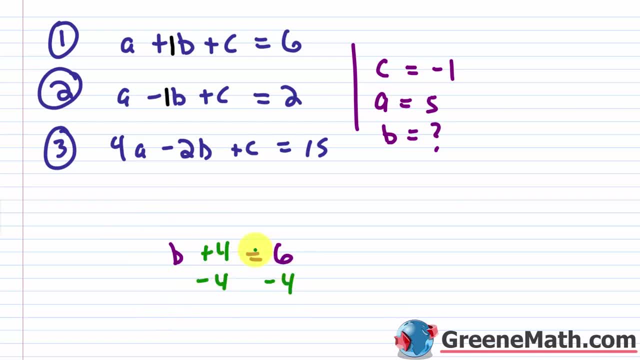 And I'm going to go ahead and just subtract 4 away from each side of the equation and find that b is equal to 2.. Okay, so b is 2.. Alright, so let's grab these values and go back up. Okay, so plugging back. 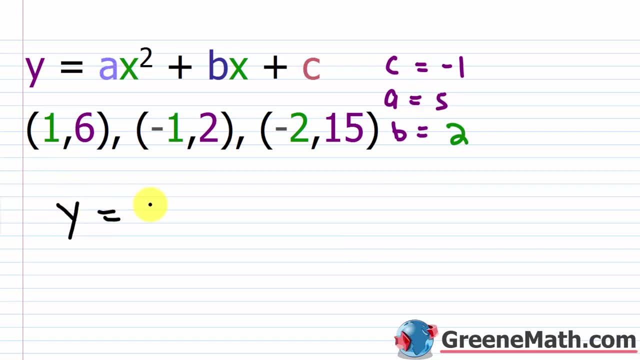 in here we have: y is equal to. For a, we have 5.. So 5, and then you have your x squared, And then plus for b we have 2.. So times x, And then for c we have negative 1.. So minus 1.. So the equation of: 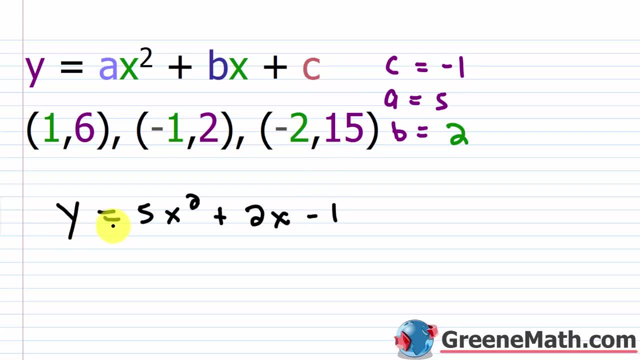 the parabola that passes through these three points would be: y equals 2.. And then, for c, we have 5x squared plus 2x minus 1.. Again, you could check this. You could take these points, plug them in. 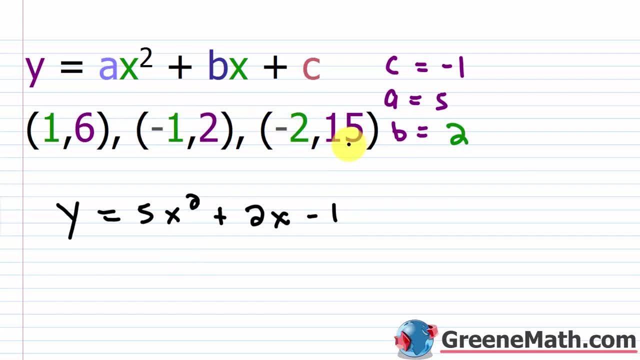 and see if you get a true statement. You should. for every scenario, I advise you to pause the video and check. I've already done that. I know this is the correct solution. Alright, let's look at one more problem, And for this one I'm going to kind of give you a spin on this. Suppose you, 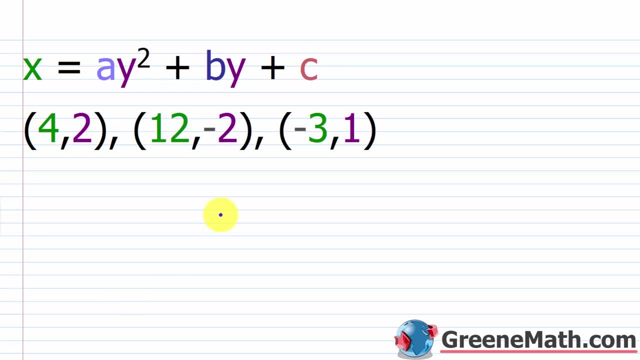 have a sideways parabola. Okay, you know, if you get something like x equals y squared, This is a sideways parabola, Okay. so what you're going to do is you're going to take this and you're going to do the same thing. So we have x equals, We have ay squared plus by plus c, And we have three points. 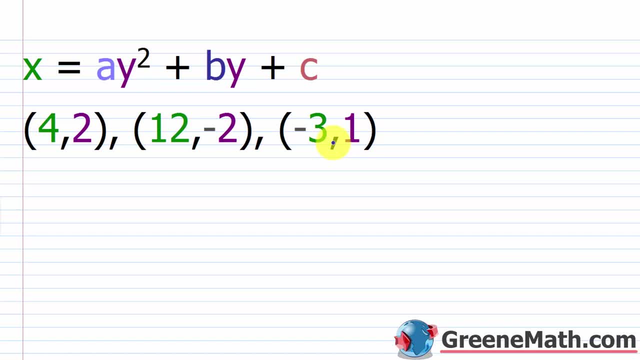 that are on this parabola, This sideways parabola. Okay, so we're going to solve and figure out what this equation is going to look like, The parabola that goes through these points. Again, this one's going to be a sideways parabola, So I'm going to do the same thing, But I've got to kind of change. 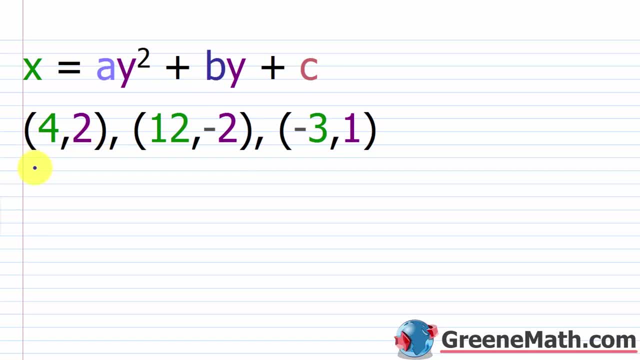 up what I do. Normally I take my y value and put it out on the left, But now I'm going to take my x value and do that. So I'm going to take this x value and put it out on the left And I'm going to 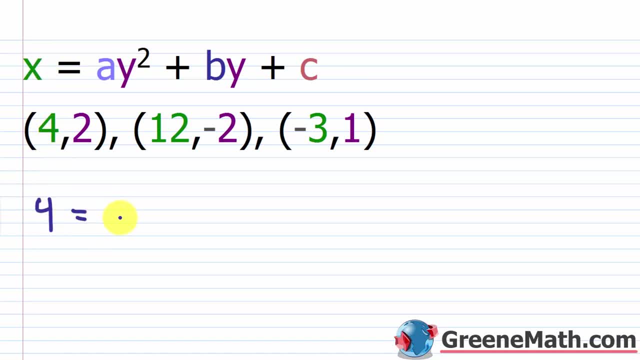 take my x value of four. Okay, because x is on the left here, This equals You have a times For y. I'm now going to plug in a two. Okay, that's going to be squared. And then plus b times for y, I have 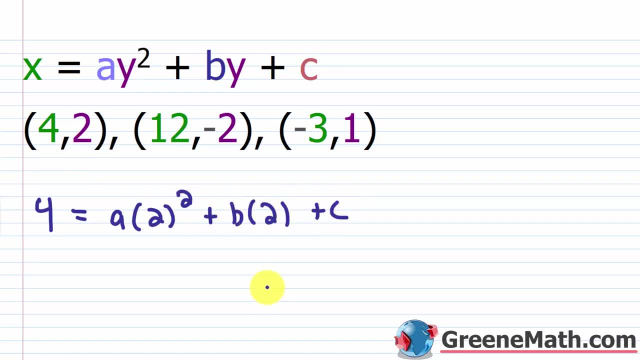 a two again, And then plus my c. Okay, and I'm going to do this again. So I'm going to have my 12. That's my x value Equals a times I've got my negative two. That's going to be squared Again. 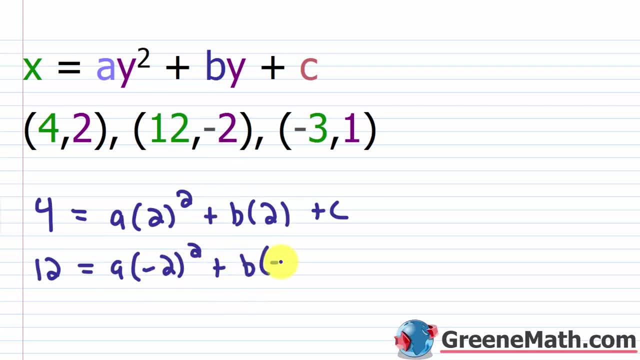 that's my y value, Then plus, I've got b times my negative two And then plus c. Okay so you're just switching what you're doing Normally: you have your x's going here and here And your y here. Now that's flipped Right. now your x goes over here, Your y goes here and here. Okay so, 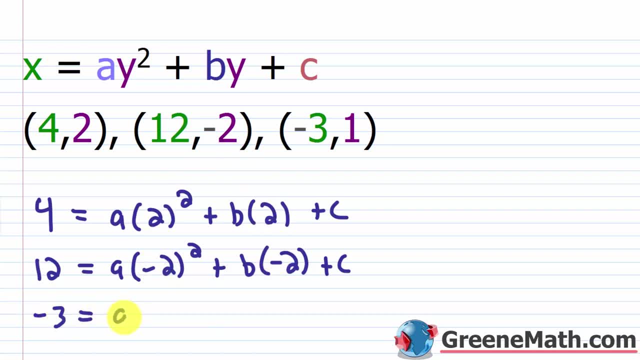 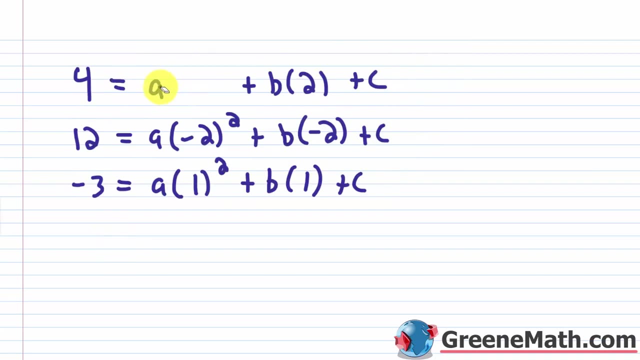 one more. We have our negative three. that goes here. This equals a times Again. plug in the y here. So one squared, Then plus b times one And then plus c. So let's copy this. We'll come back up, Get a nice fresh sheet going Again. two squared is four, So this would be four a, So let's put four. 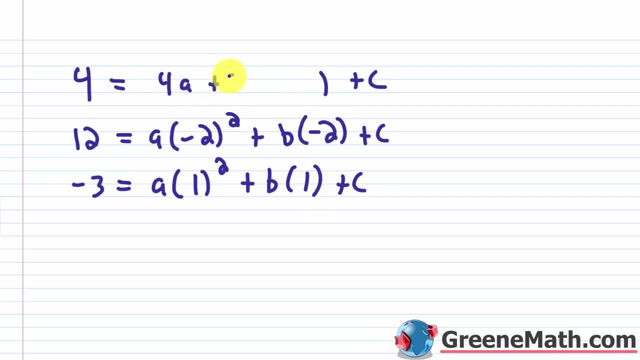 and then two times b is two b. So plus two b Plus two b, And then plus c. Okay, so plus c, And let me put equals four on this side. I can erase it from here. Let's go ahead and just label. 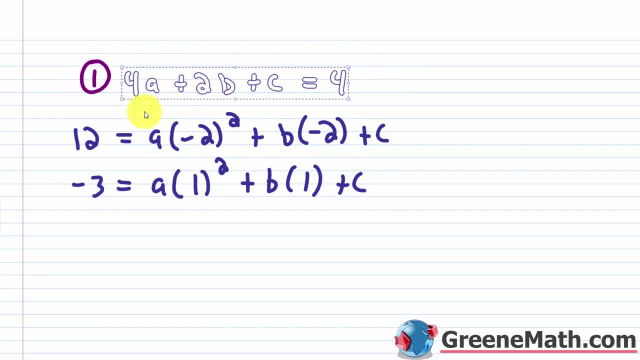 this as equation one. Okay, let me kind of slide this down, Save a little room, And we'll slide this down a little bit more. Okay, so for the next one: negative two squared is going to be four, So we'd have four a And then negative two times b is minus two b, So we'll put minus two b And then. 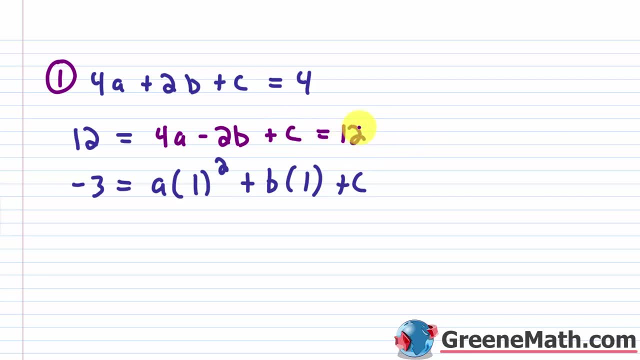 let's put plus c, And of course this equals 12.. We'll just erase it from over here. So this is going to be equation two. Let me just kind of slide this one down. Okay, so one more to do. So we have one squared, which is one. You just get rid of that. One times b is just b, So you get rid of. 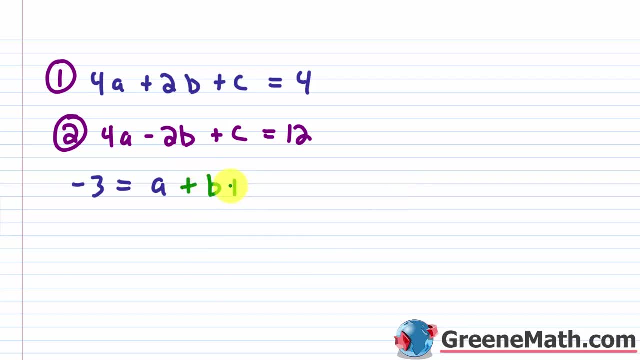 that. So you have a plus b plus c. So a plus b plus c, And this equals negative three. So let's get rid of this, Let's put this as equation three And let's slide this down. Okay, so what variable? 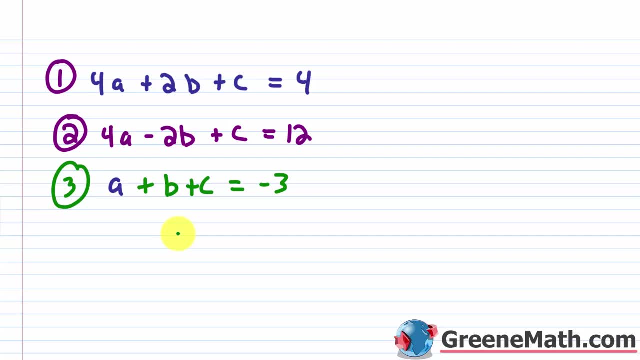 eliminates. Again, it's pretty easy to do b. It's also pretty easy to do c. A looks like it's a little bit more work, But even that's pretty easy. So let's just go ahead and eliminate the variable b, So I can go through with the first two equations And I can just add them. Okay, because 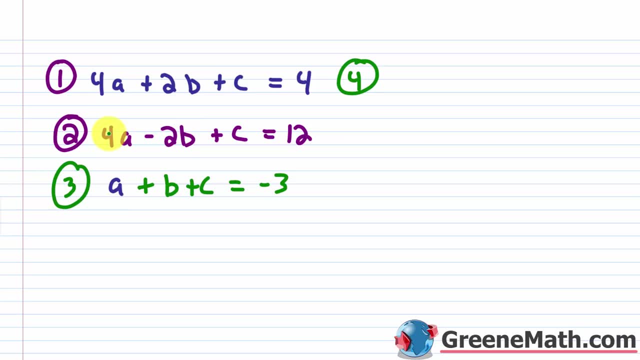 I have two b and negative two b, So four a plus four a is eight a. So this is eight a And then two b plus negative two b. That's going to cancel, And then c plus c is two c And then four plus. 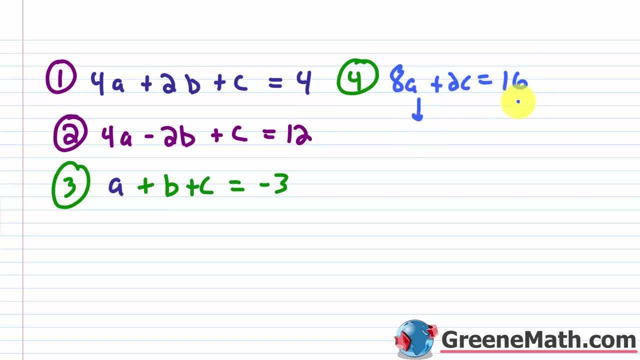 16.. Again, I can simplify this: Divide each part here by two. A divided by two is four, So four. a plus two divided by two is one, So just c, And this equals 16 divided by two is eight. Okay, then for equation five. Let's get that from two and three, Okay. so what I'm going to do is I'm 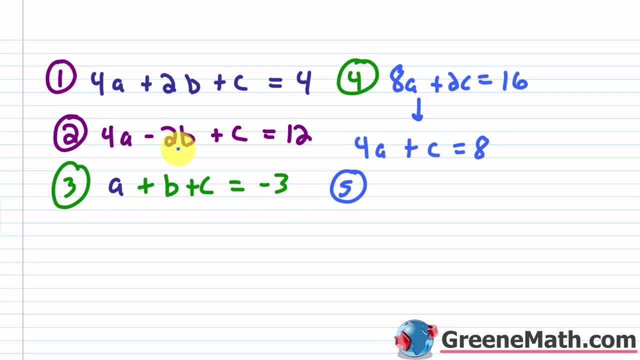 going to multiply equation three by positive two, So that I can have opposite coefficients on that variable b. Okay, so if I multiply equation three by two, I'd have two a plus two b Plus two c equals negative six. Again, I just multiplied everything by two, Then I keep. 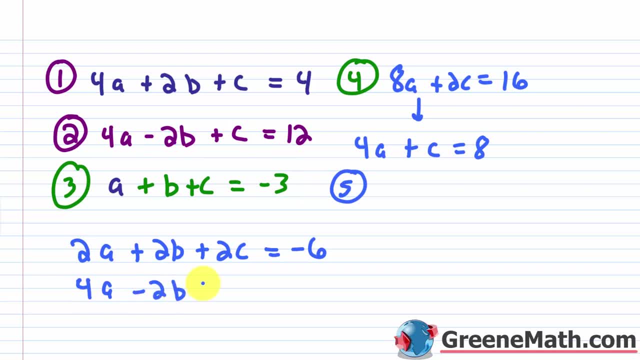 equation two as is. So four a minus two b plus c equals 12.. Okay, so let's go ahead and add the left sides. Set this equal to the sum of the right sides. Two a plus four a is six a, Then two b minus. 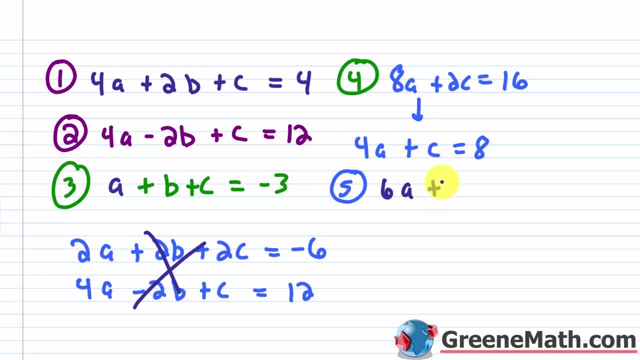 two b, That's gone. Two c plus c is plus three c, And then negative six plus twelve is six. Okay, so again we see that we could simplify this. We could divide each part by three, So this would be: two a plus c equals two. All right, so let me erase this and write this just as: four a plus c equals eight. 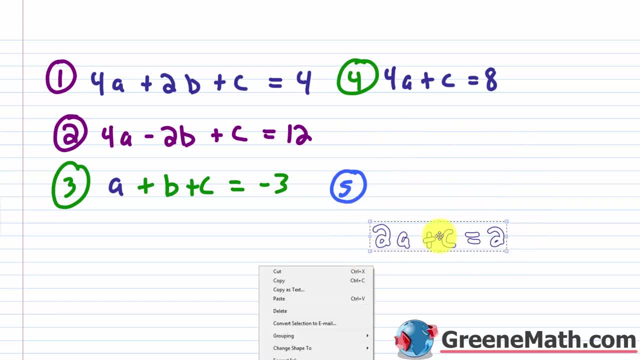 Let me erase this and just kind of drag this up Again. it's two a plus c equals two. So we can just use substitution here. I know that I can solve this guy for c. I say c is equal to Subtract two a away from each side. So negative two a plus two. 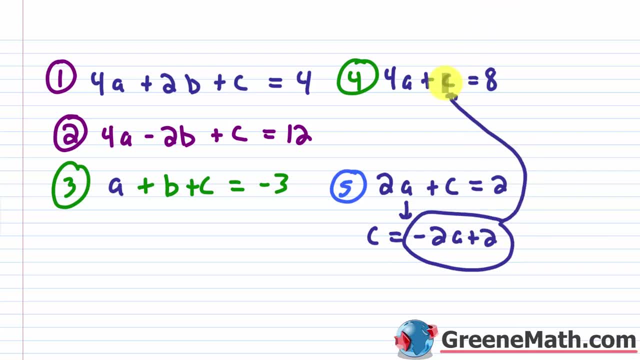 And then plug this in for c here. Okay, that's all I'm going to do, Plugging this in, because c is equal to this in there. So what we're going to have is that four a plus We'll plug this in for c. So 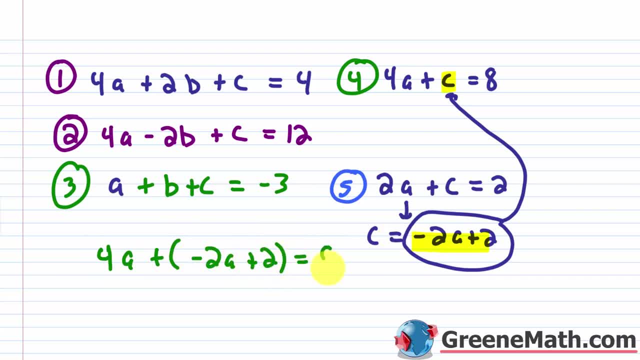 negative. two a plus two, And this is equal to eight. Okay, so I can just drop these parentheses. They don't really do anything here. So four a minus two a is just going to be two a, And if I subtract two away from each side, this would go away and this would be six. 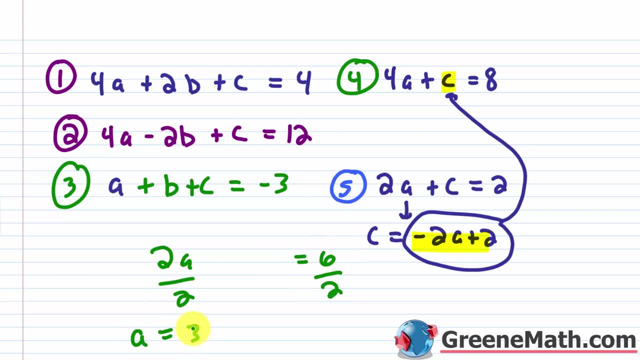 And I'm going to find that a is equal to three. Okay, so a is three. I can erase all this and I'll just write that over here for now. So a equals three. Plug that in in equation five. Plug in a three. there You'll see that two times three is six. So six plus c is equal to two, If I subtract. 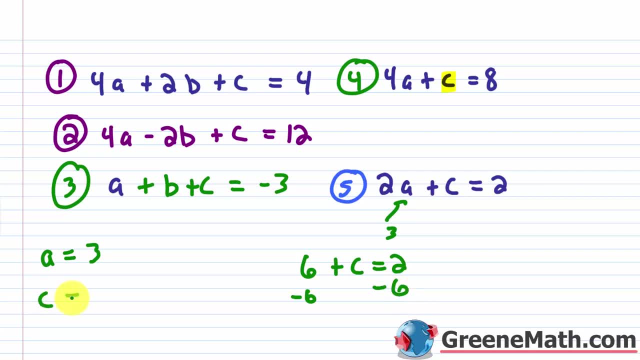 six away from each side of the equation, I'll find that c is equal to two minus six is negative four. Okay, so let's erase these. We don't need this information anymore And we're just going to write this up here and say that. 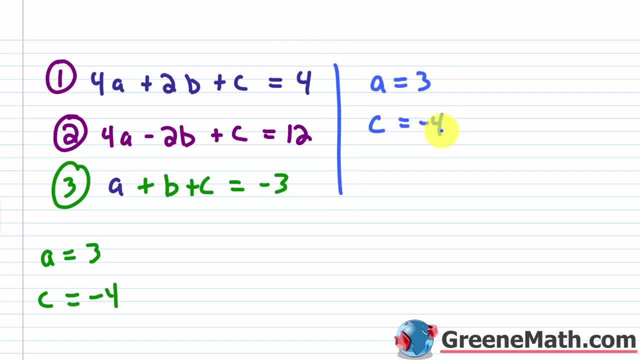 a is equal to three and c is equal to negative four. Let's erase this. And now let's just go ahead and plug in and find out what b is. So b is our unknown, So let's plug into equation three. That's the easiest. So I'm going to plug in a three there. I'm going to plug in a negative. 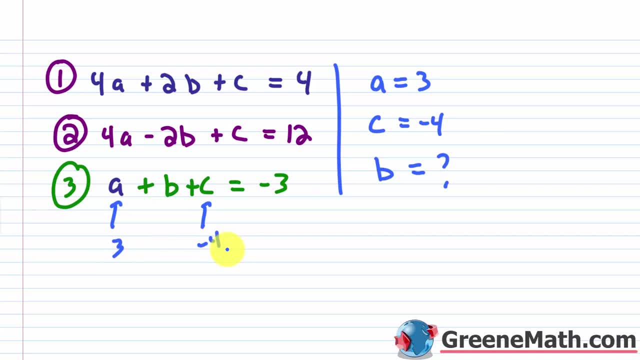 four there. So I already know that three minus four is negative one. So let me just write this as b minus one equals negative three. Add one to each side of the equation and I'll find that b is negative four. Okay, so let's put a negative two there And let's just copy this real quick. 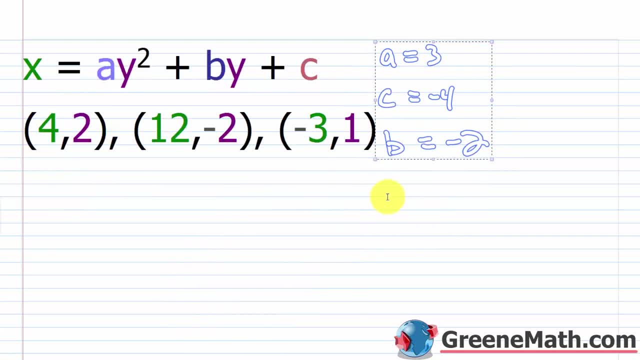 and go back up. So we'll copy these values. Okay, so let's go ahead and write our equation. So we have x. now, Remember this is different. This is a sideways parabola, So x is going to be equal to: for a, we have three, then times y squared, Then plus for b, we have negative two. So let me just 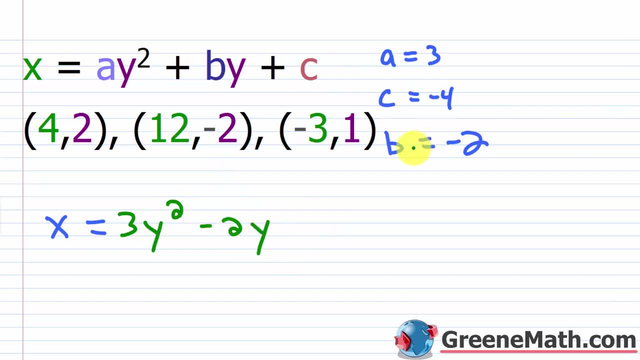 write minus two, So minus two times y, And then for c we have negative four, So minus four. Okay, so x equals three, Y squared minus two, y minus four. So you just want to pay close attention to the problem they give you. This is much less common, but you might get it. So just pay attention to the equation you 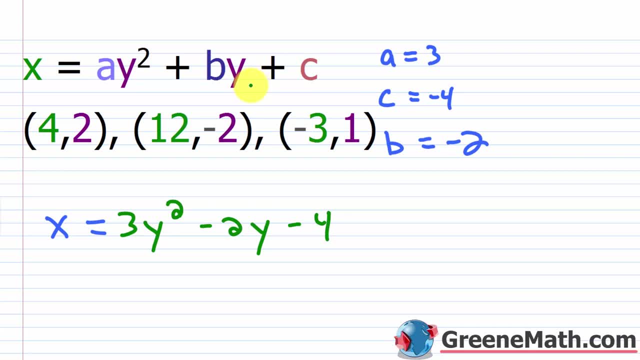 get. If you're told that the three points lie on the parabola and the equation is: y equals ax squared plus bx plus c, Do what we did in the first two problems. If you get a sideways parabola again, like this one where x is equal to ay squared plus by plus c, Again, you want to follow this.